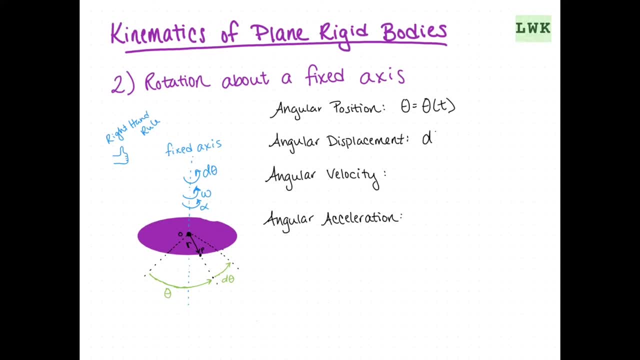 displacement, therefore, is going to be defined as d theta. So that's going to be our change in angular position. So now, like we've done many times before, we're going to say that our angular velocity is going to be the derivative with respect to time of theta. 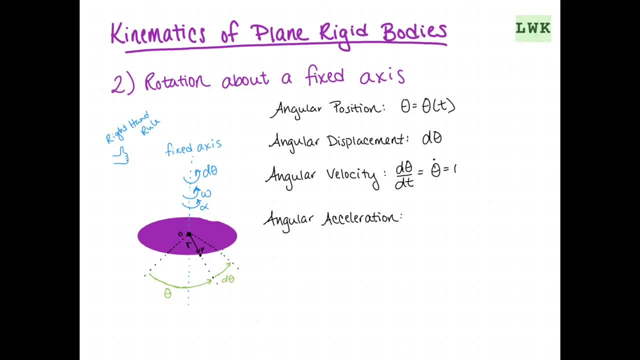 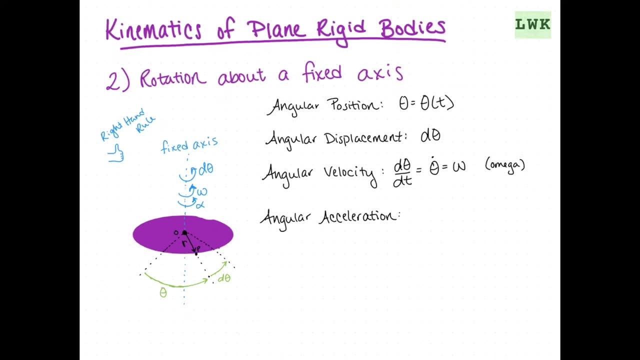 And we could write that as theta dot, But going forward, we're going to use omega to designate our angular velocity And of course we can say angular acceleration. we can write as d two theta over dt squared or theta double dot, But we're going to say, going forward, alpha is going to be. 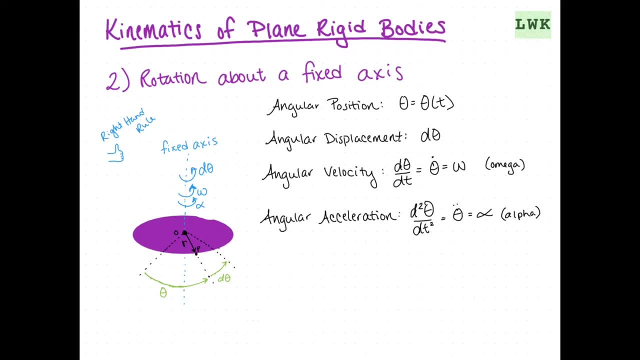 designating our angular acceleration. Now, another important thing to note is that any line on the body is going to have the same angular velocity and acceleration, And we also can say that our alpha here is equal to omega d, omega over theta. That's just another way that we can define alpha. 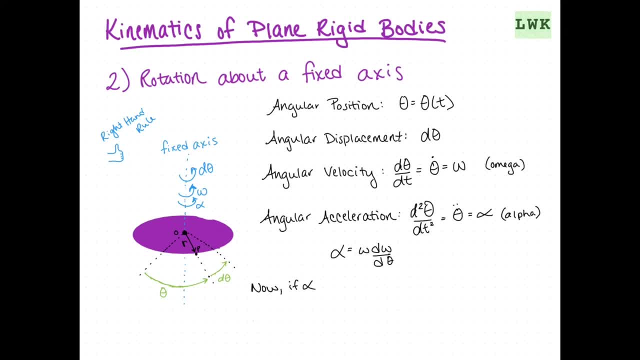 Now it's going to be a function of time. So we're going to say that our angular velocity is going to be: If alpha equals a constant, we can use a certain set of equations So we could say: and these should look pretty familiar. And another important thing to note is that these problems are really set up. 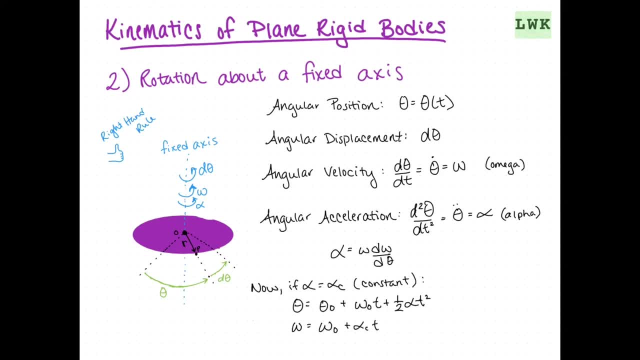 ideally for polar coordinates. So that's kind of where we're going to be drawing from. So we're going to So the molarStar and the diagonal, as you're going to see in a moment. So far we've drawn from an anchor that we're going to be Pakistanため, type of solution for Euler's. 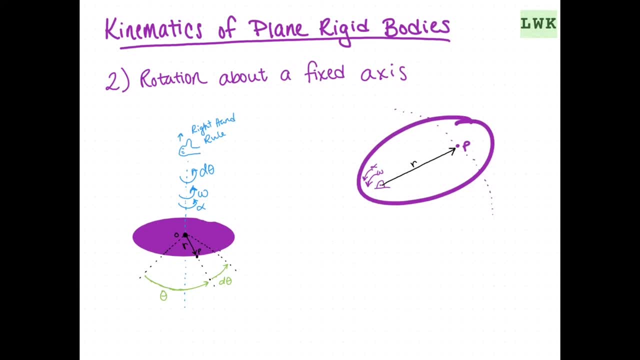 a constant acceleration. So now you can see here we've drawn another sketch on to the right And this is as if we're looking down on this plane rigid body. So you know, our axis will be pointing up at us And we pretty 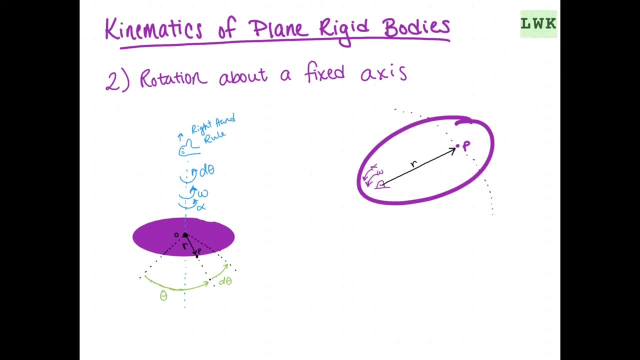 much drawn the same situation that we have on the left. So what happens now if we want to find the velocity of this point, P? So again, we know that any point that's rotating about a fixed axis is going to have a circular path of motion. So we know that P is going to be moving in a circle. 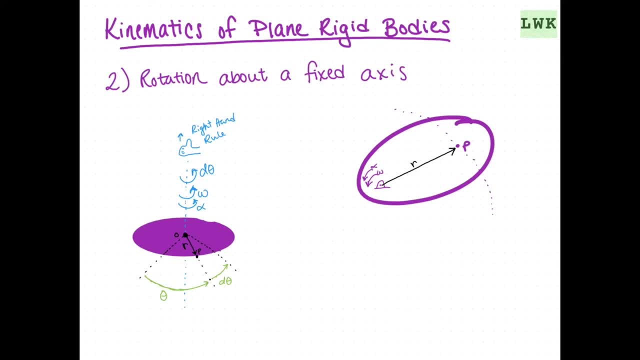 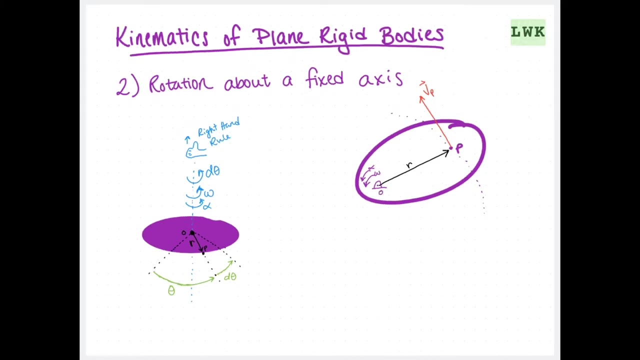 So we can say that our velocity is going to be perpendicular to this line R, and we'll call it VP, And it's going to be tangent to our path of motion. So we can write an expression for VP and we can say: VP is going to be equal to R times omega times U sub theta. And we have essentially, we derived this from the equation. So we can write an expression for VP and we can say: VP is going to be equal to R times omega times U sub theta. So we can write an expression for VP and we can say: VP is going to be equal to R times omega times U sub theta. 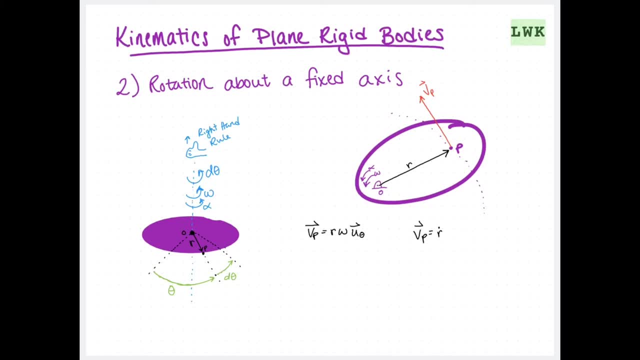 Because we can say: VP equals R dot U R plus R, theta dot U theta, And this is going to become zero because R is going to be a constant. So VP is going to end up being equal to R theta dot U theta And, as we just defined, theta dot is going to be R omega. 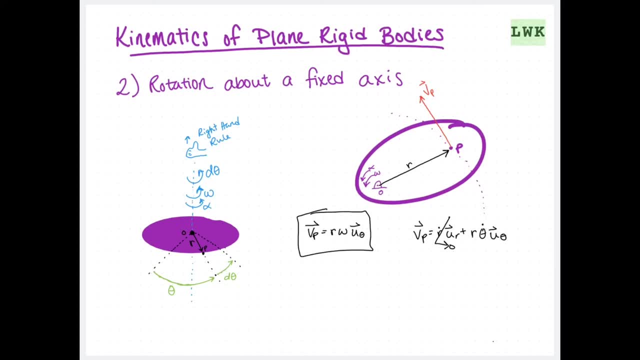 So here is our VP expression, and if we want to say you know the magnitude vp, we're going to write that as omega times r. so now, if we want to write our acceleration of point p, we can say: ap equals r, double dot minus r, theta dot, squared u r. and again, this is just you know what we know. 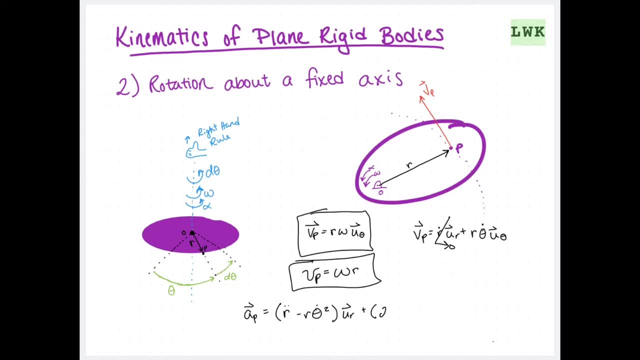 from our polar coordinates from our previous lectures. so times two, so theta, and again with r being constant. so This is going to be equal to 0, and this is going to be equal to 0.. So let's write this out again: This is going to be equal to negative. r theta: dot u sub r plus r theta- double- dot u sub theta. 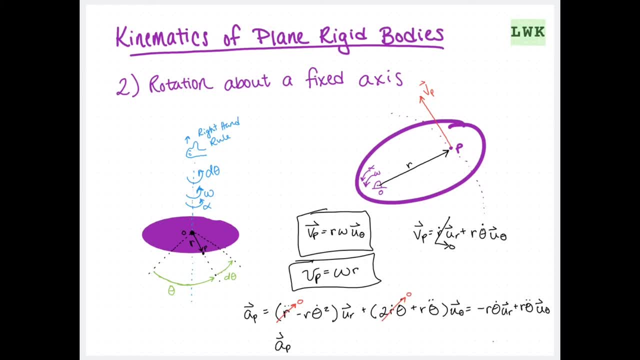 So our final expression for the acceleration of point P, we can write that as negative r, omega squared times u sub r. So that's our r component plus our theta component is going to be equal to alpha times r. So that is our final expression. 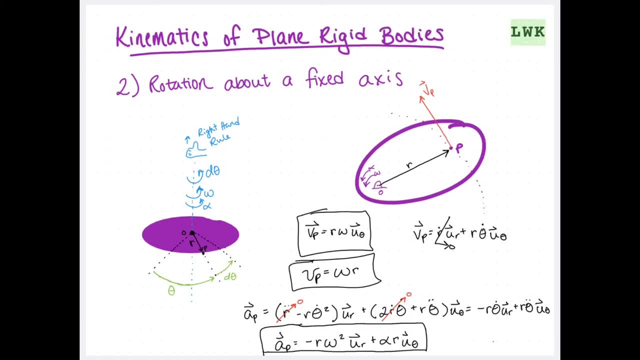 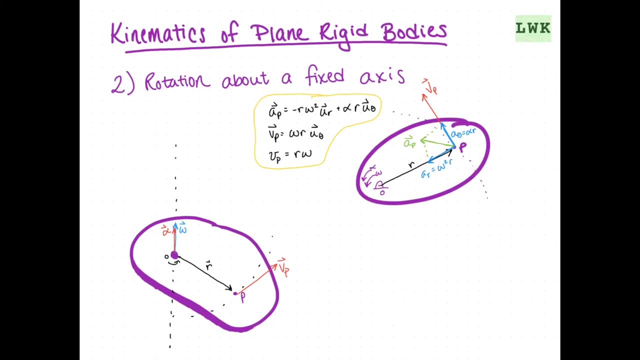 For our acceleration at point P. So here in our top right we've drawn in our r and our theta component of our acceleration And we have created in green our resultant vector, so a sub p, which is going to be expressed by our equation in yellow that we just defined. 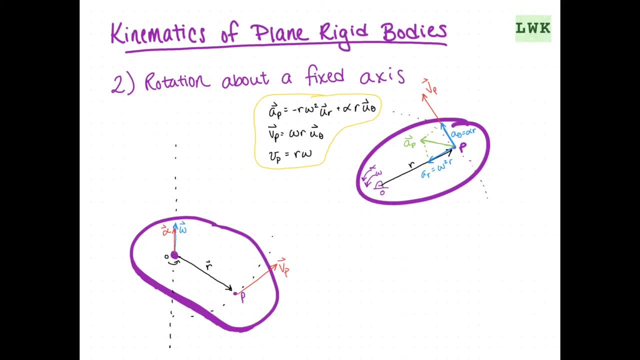 So now, if we look in our bottom left, we have essentially the same picture, but we're going to look at it from another angle. And we're going to look at it from another angle. So now, if we look in our bottom left, we have essentially the same picture, but we're going to look at it from another angle. 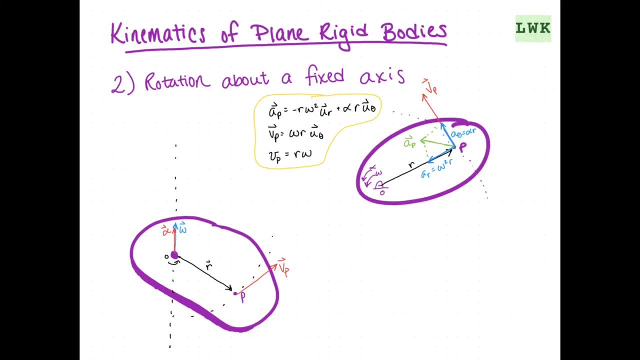 And we're going to define all of these values using vectors. So we could write v sub p as equal to the cross product of omega and r like so, And, as you can see on our picture we have, omega is pointing up in the same direction of our axis. 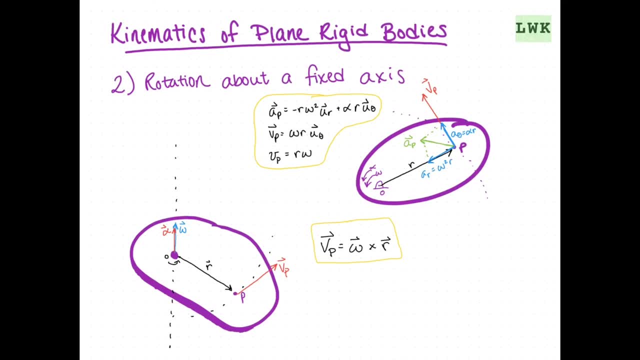 And we have essentially all of these values And we have essentially all of the same components as we did before. So this is going to be how we write as vectors omega cross r And for our acceleration we can say: this will be equal to alpha cross r plus omega cross omega. 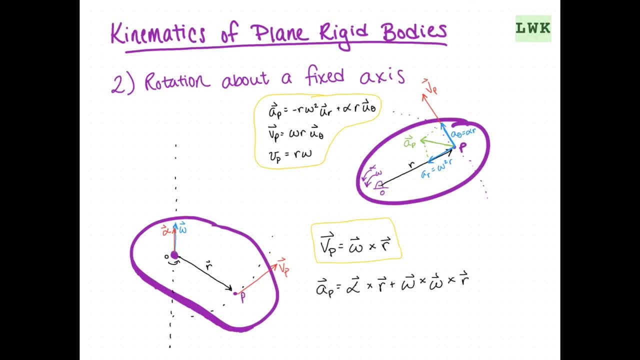 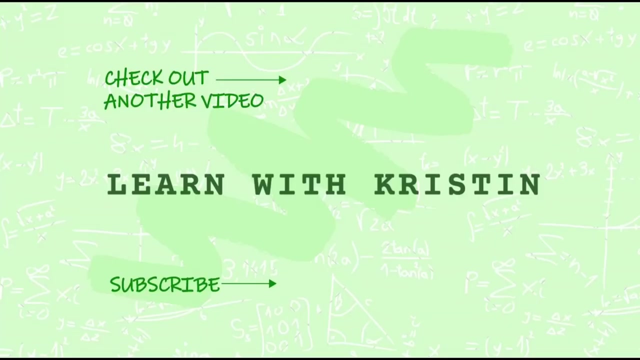 Or we could write it a little simpler as a sub. p equals alpha cross r minus omega squared r. Thank you for watching. If you like this video, please be sure to give it a thumbs up and subscribe. That really helps support my channel. 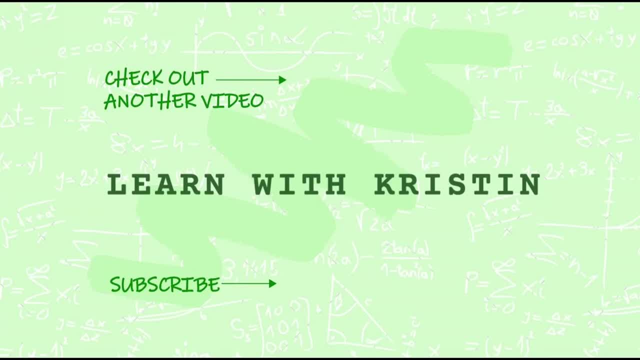 And helps me continue making videos for you guys. I'll see you next time.